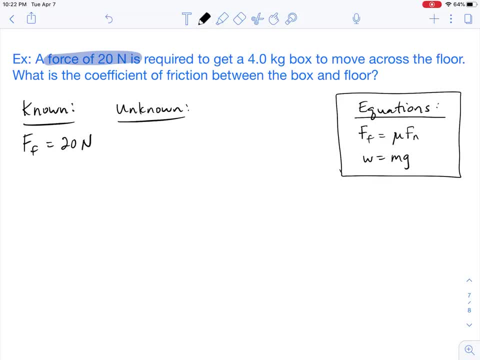 then that would be our kinetic friction or our coefficient of kinetic friction. All right, so we have our force of 20 newtons. We also have a four kilogram box, So that would be our mass, four kilograms. And once again, what is the coefficient of friction? That's what we are solving for, So we 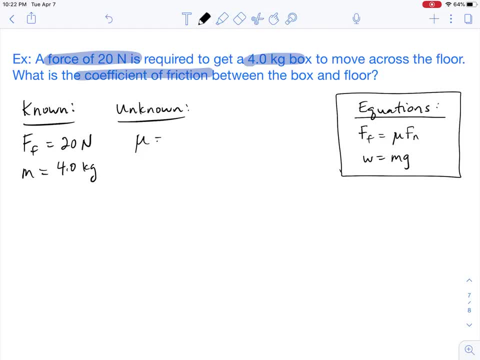 are finding our mu value. So that's what this little letter is. It's a Greek letter called mu and it represents the coefficient of friction. So with these force problems, I always recommend drawing a free body diagram. Draw your picture that shows all the forces that are acting. 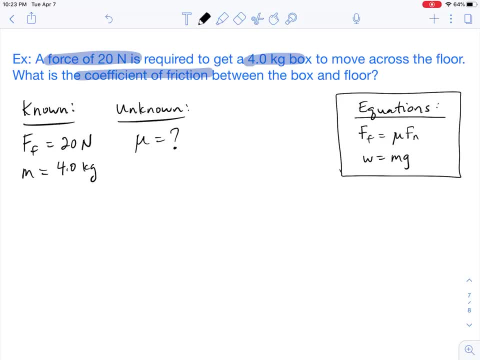 on your object. That's going to help you figure out how to use the correct equations and get your answer. So basically, we have a box. Once again, the box is on the ground. We know that gravity is always acting on our objects, So that's our weight force. So weight equals mg. 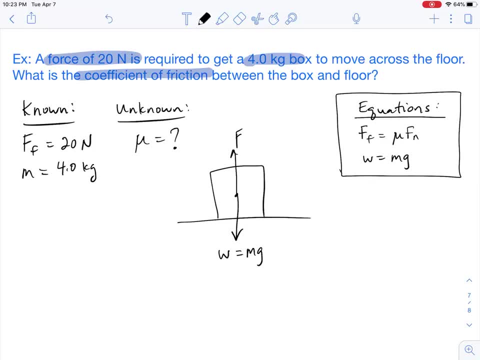 The surface is pushing up on the box. We call that the normal force, And then we said that a force of 20 newtons- so I'm going to say it's being pushed to the right- is what overcame our friction force. So in that moment, 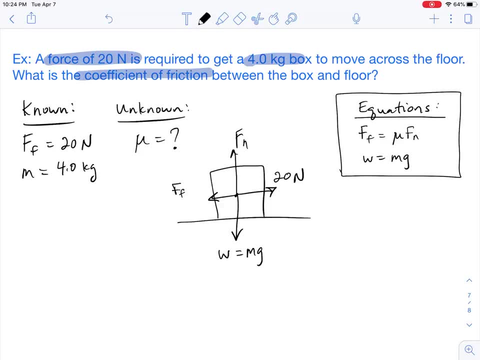 the friction force was also 20 newtons. We were able to overcome that with 20 newtons of, So we'll just label that the friction force as well. All right, So how does this free-by diagram help us? Well, if you take a look at our equation, the equation that we need to use looks like this: 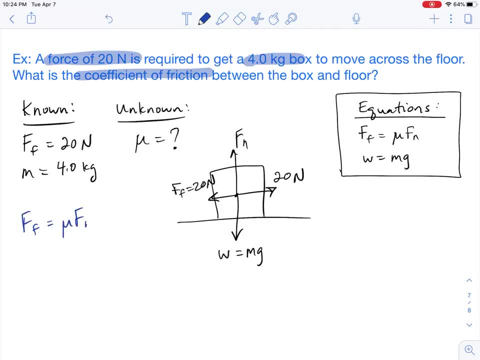 Friction force equals mu- Fn. So mu, our coefficient of friction, times our normal force. Our normal force isn't listed in our known value, though, So how are we going to get this normal force right here? Well, it turns out that, according to Newton's third law, for every action there's an equal and opposite reaction.